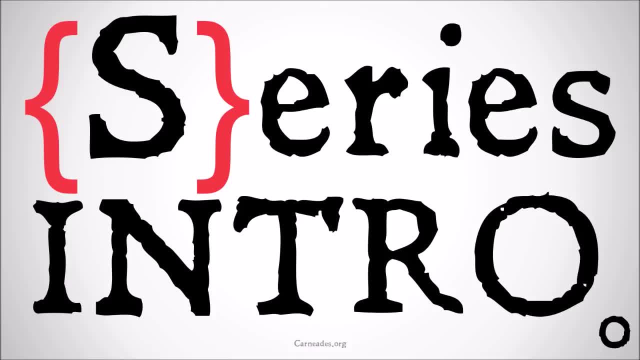 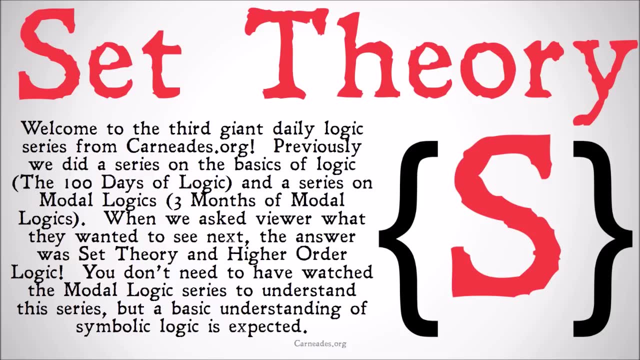 Now this is just going to be a quick series intro. Later today we're going to be putting up another video and then we're going to be going for the whole month of October. a video every single day on set theory. So welcome to the third Giant Daily Logic series from Carnity80sorg. Previously we did a series on the basics of logic That was called the 100 Days of Logic. 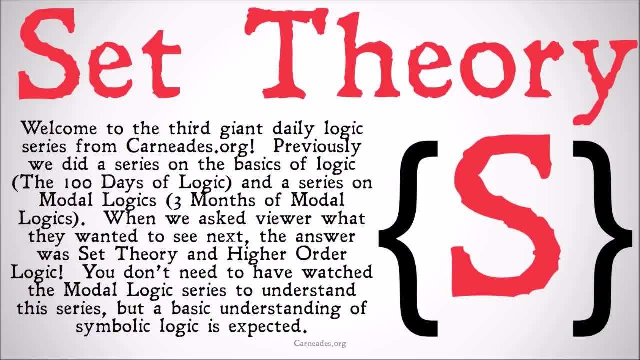 Then we did a series on modal logics- three months of modal logics. When we asked viewers what they wanted to see next, the answer was set theory and higher order logic. You don't need to have watched the modal logic series to understand this series. This series is not really going to build on anything in modal logic. 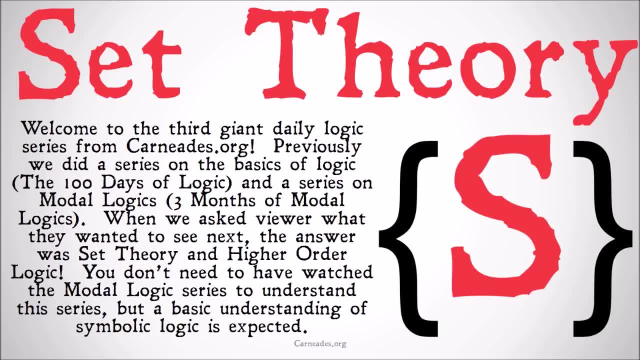 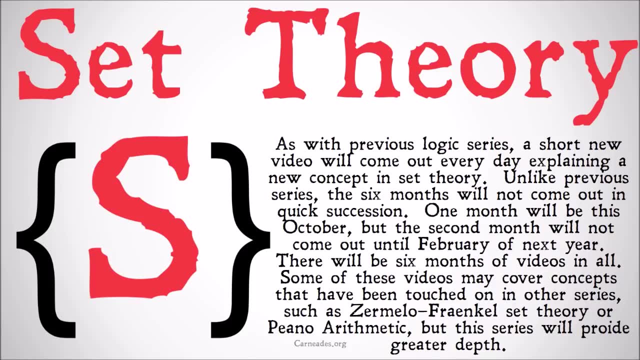 We're not using that, using modal logic, much of it all- but a basic understanding of symbolic logic is going to be expected. it's an understanding that you can get from watching the 100 days of logic or from taking a introduction to logic course at most major universities. as with previous logic series, 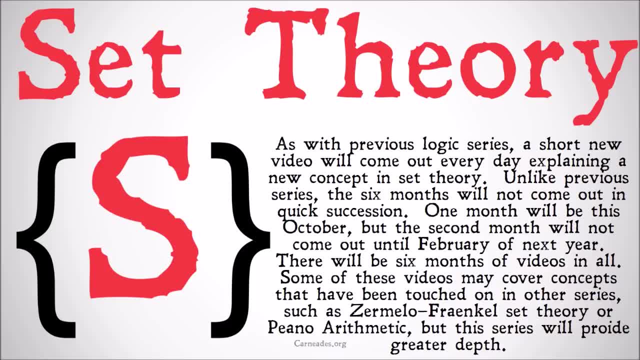 a short new video is going to come out every day, explaining a new concept in set theory. unlike previous series, though, the six months aren't going to be right after one another. i can't make that many videos, and you'd probably get tired of it. what's going to happen is we're 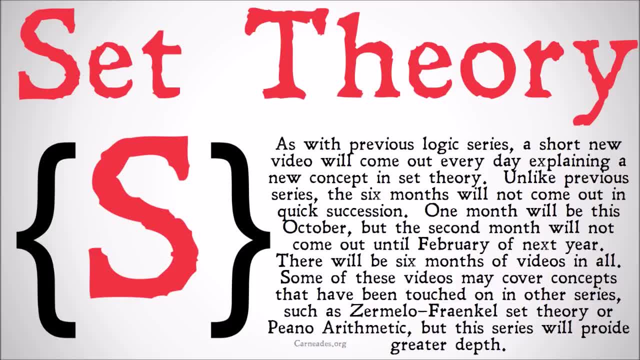 going to put one month out in october, this month, and then the second month is going to come out in the february of next year and then future months will come out in later months, maybe october of next year, depending on how much time i have to make these videos, because these series 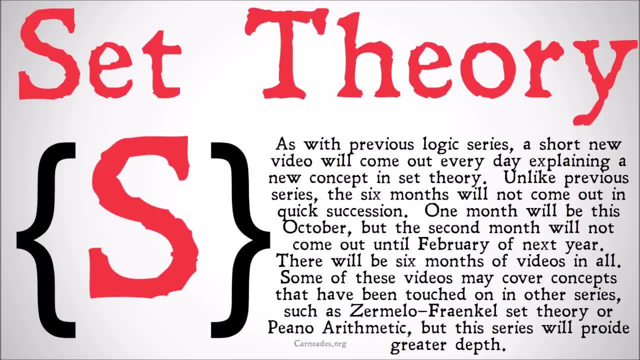 take a lot of time and work. there's going to be six months worth of videos in all, because there's a lot to cover within set theory and higher order logic. some videos may cover concepts that have been touched on in other series, such as zermelo-frankel set theory or piano arithmetic, but this series is going to provide 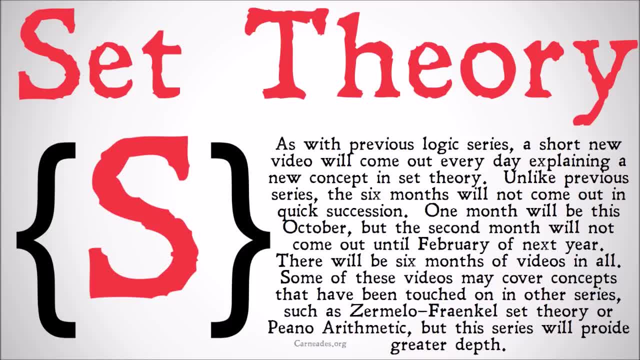 greater depth for them and it's going to hopefully provide them at a pace that even people that don't have a background in some of these things can start at the beginning of the series and go straight to the end without having to use other resources or look things up. okay, the first month.